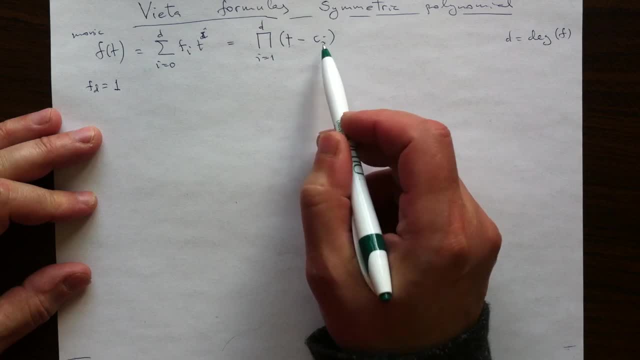 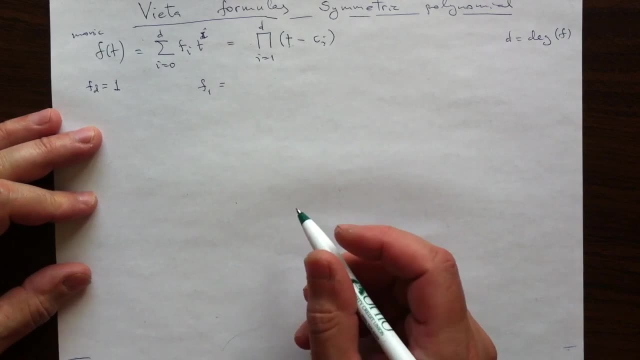 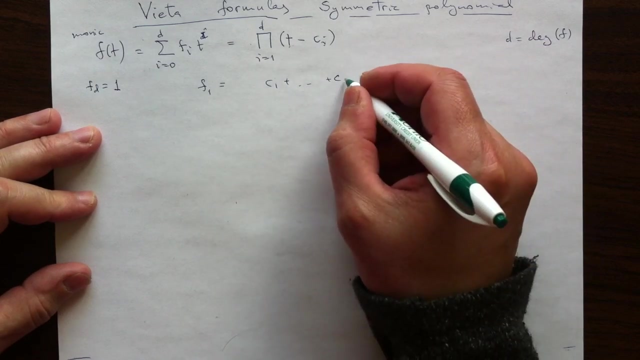 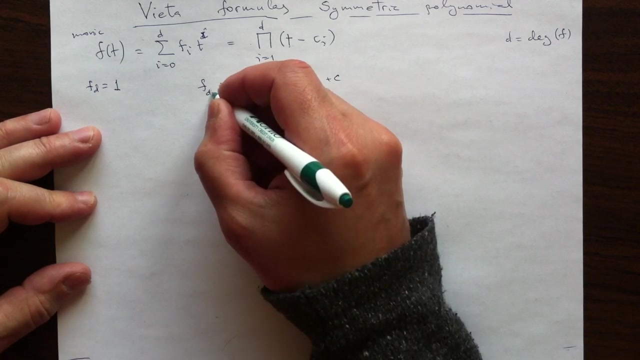 one of the factors and taking roots from all the others. and in this expansion, in the process of expanding this first coefficient, we will have the sum of all the roots. all of them will have to be taken. So that is not the first that 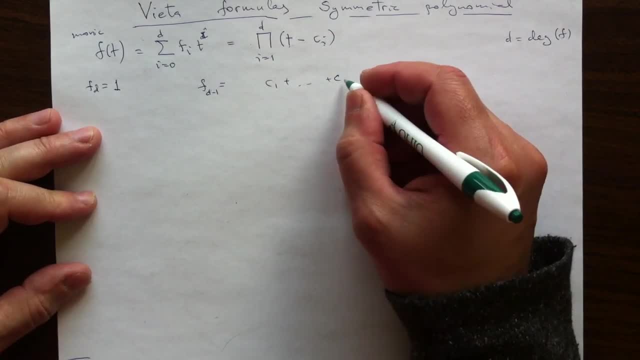 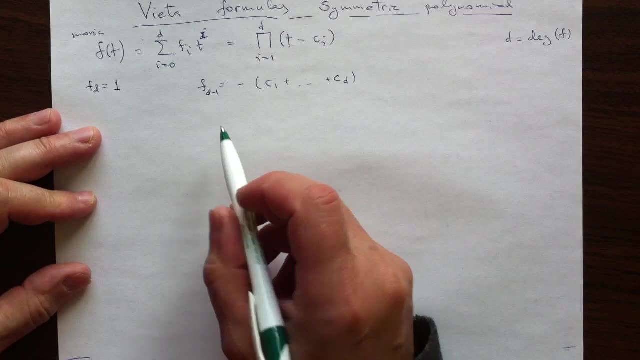 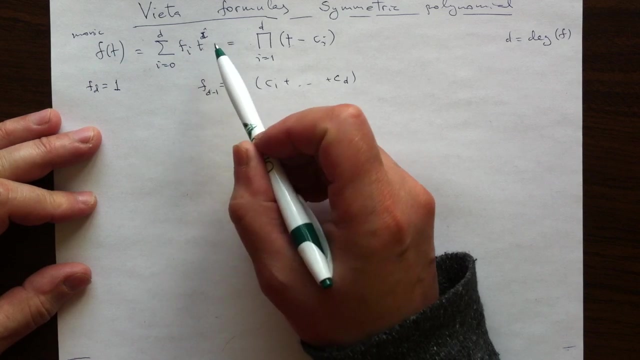 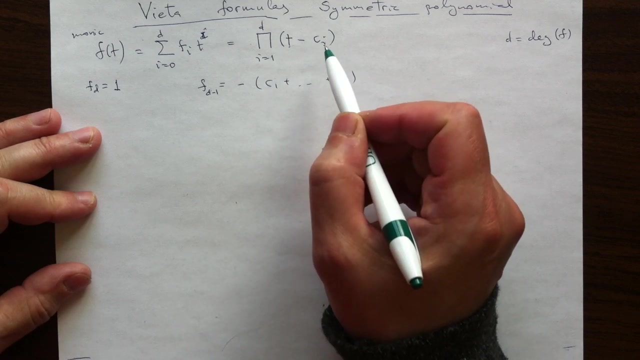 is t minus 1, it is the first after the leading, The sum of all the roots, with minus coefficient. So what I said I said incorrectly. I'm building the coefficient for the next after the leading power. so to take d minus 1, copies of t from almost all factors but one and from 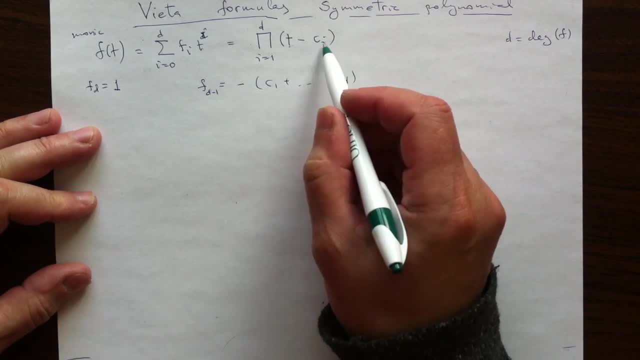 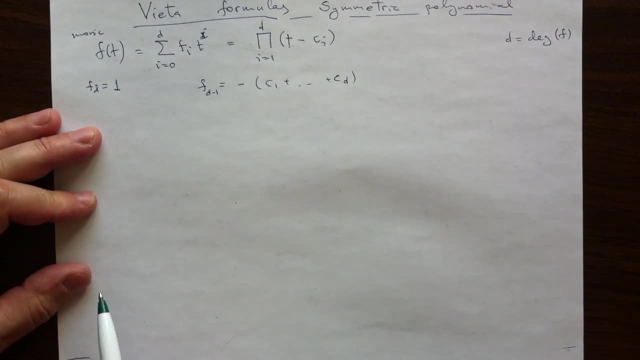 that one, I have to take the other coefficient, negative root, and then when I go through all such products, I will see this coefficient coming. So then the other extreme: when we take the other product, I will see this coefficient coming. So then the other extreme when we 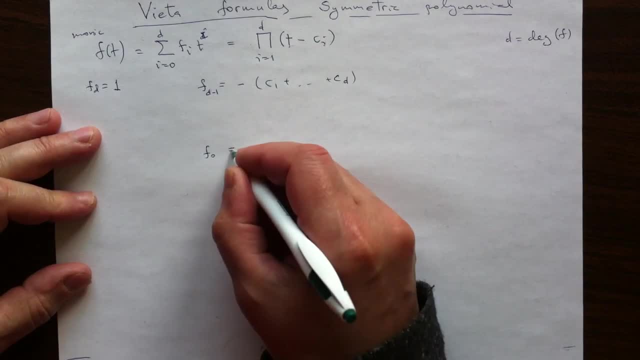 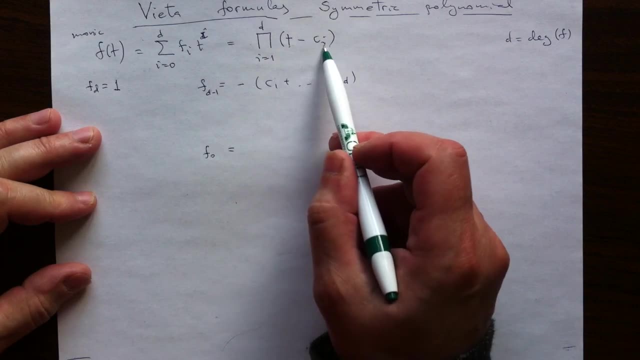 go all the way down to the free term and look at the free term, and that means that we don't have t's at all. That means that in all these products we have to choose the free coefficient root and then take the product of all of them. So 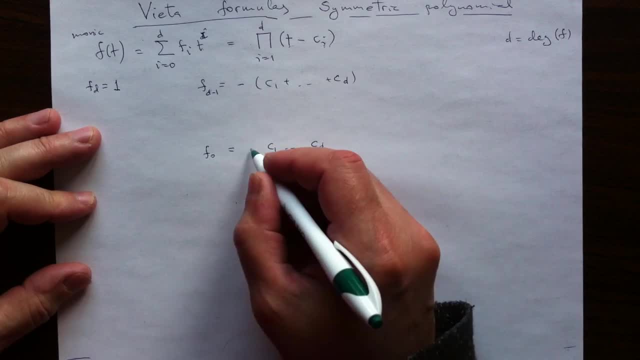 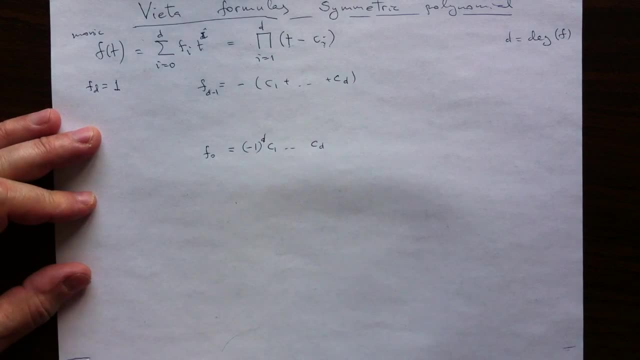 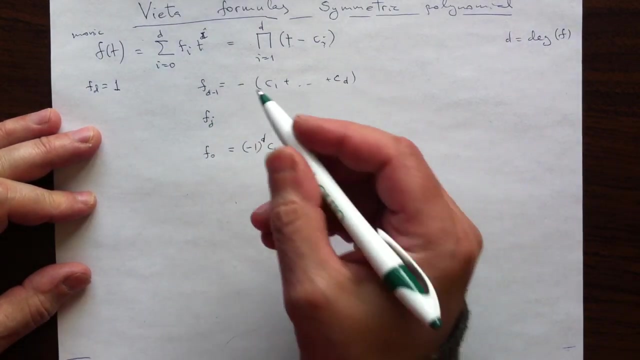 the answer will be easy: product of all the roots. but they will come each with minus sign. so the overall minus sign contribution will be to the number of those roots. So let's also recall the difference between the marginal statics. and you can see that it comes on y. 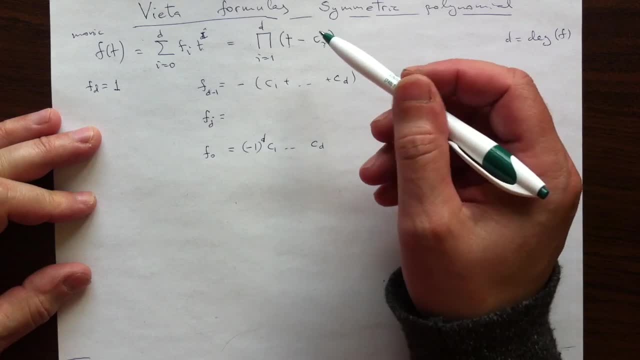 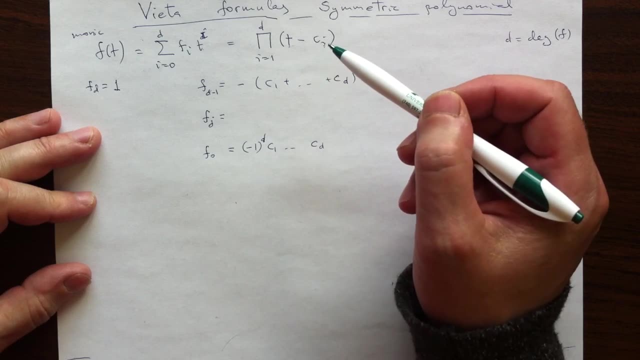 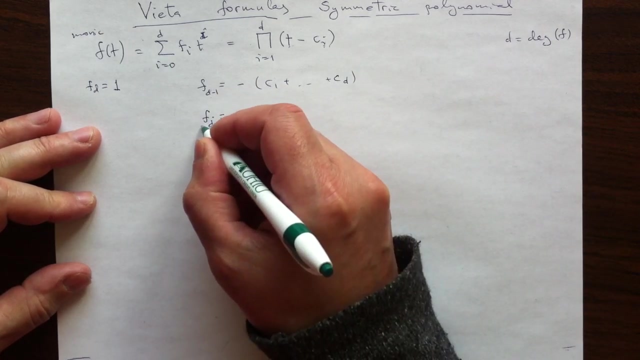 We will look at j when we look at the t to the power of j. So let's turn inside out and see what happens in between with step j, when we look at the t to the power j, And that means that we take t from j. 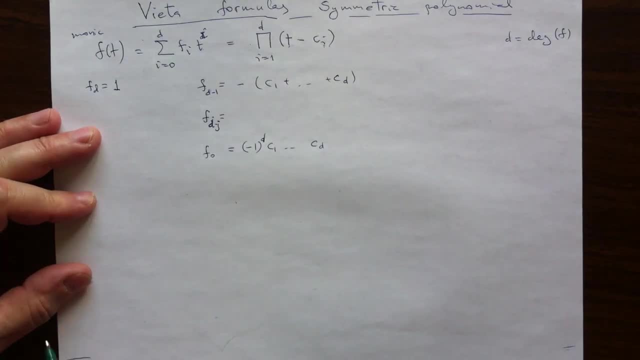 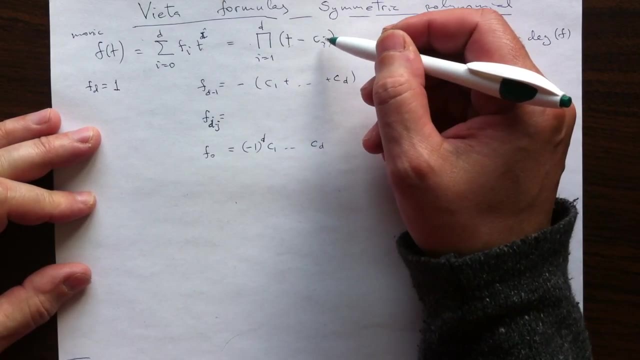 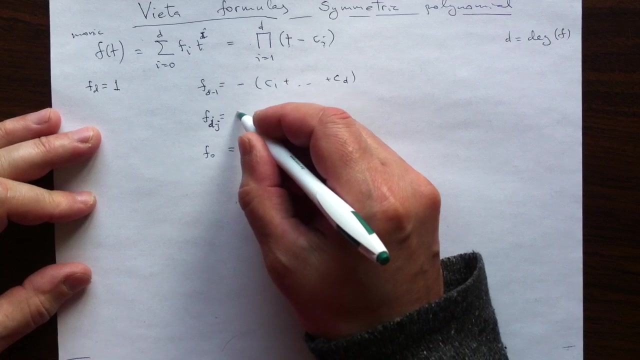 factors And from the rest we have to take the roots. So maybe I'll be better to have to take d minus j t's. so from d minus j factors i'll have to take t. from the rest i'll have to take the root. so i'll have to take j root. the number of minuses will be minus one to this. 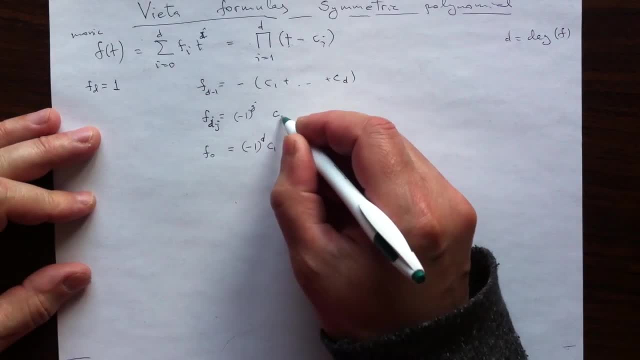 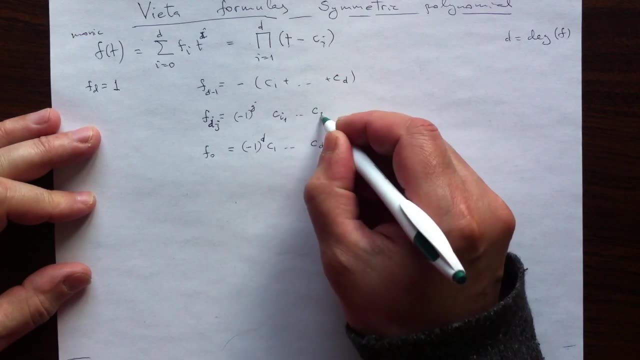 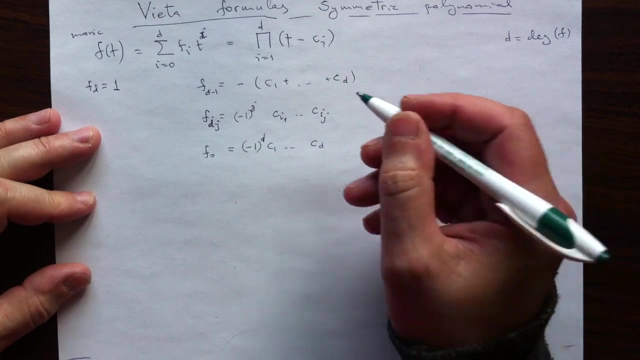 number j, and then i'll be taking some roots and since i'm going to form a product of them j such roots, they will have to be all different. i'm taking them from different factors and since i'm forming products out of them, it doesn't matter. 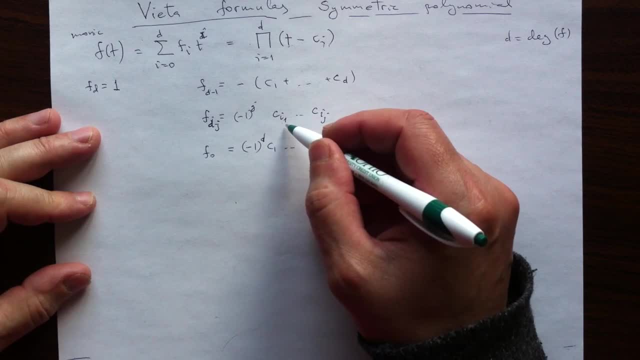 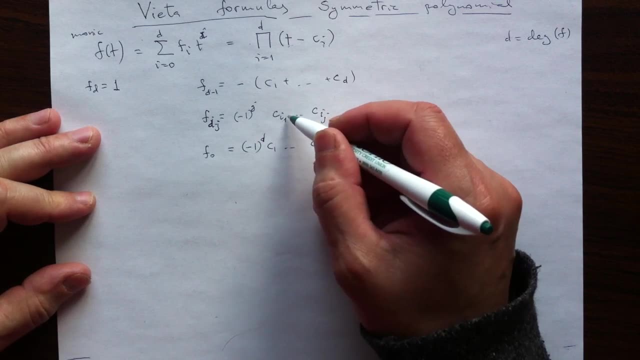 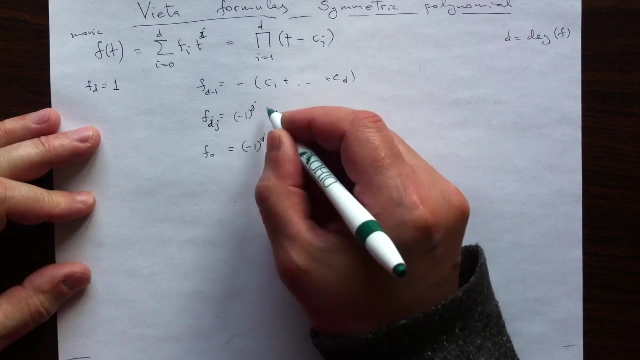 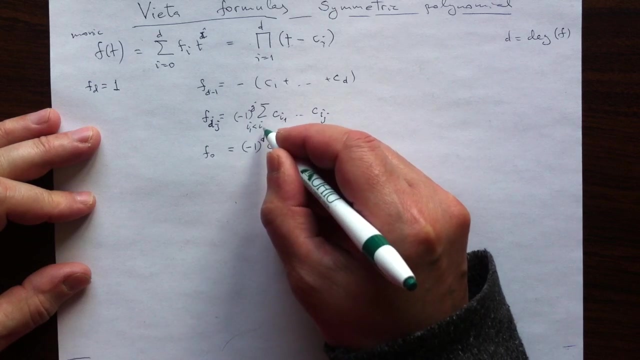 it can be made. this product can be made such that the first is index is less than the second, and so on. so i can order my roots in the product, each product, and so on. so i can order my roots in the product, each product, in such a way that the first written is its label is less than the second, and so on. 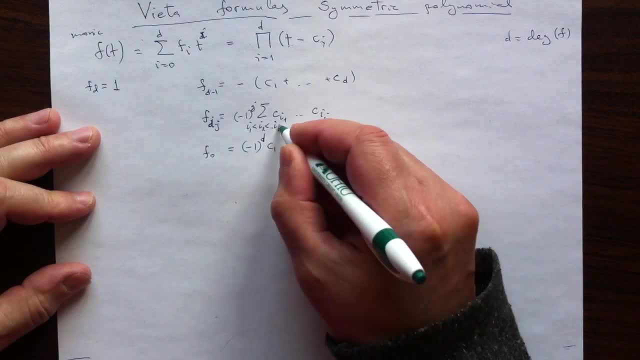 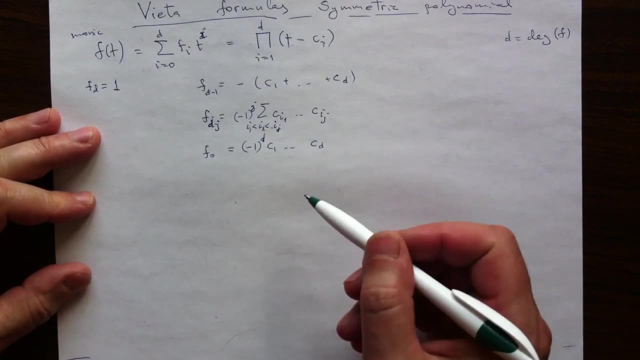 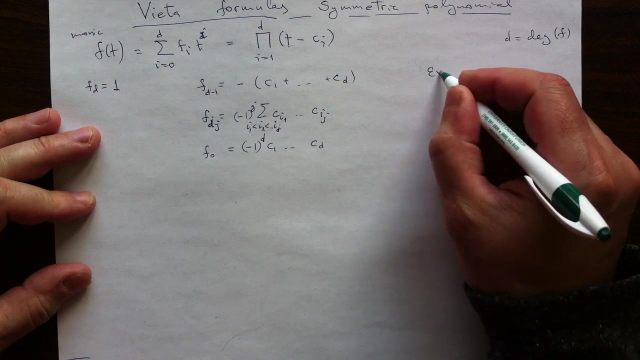 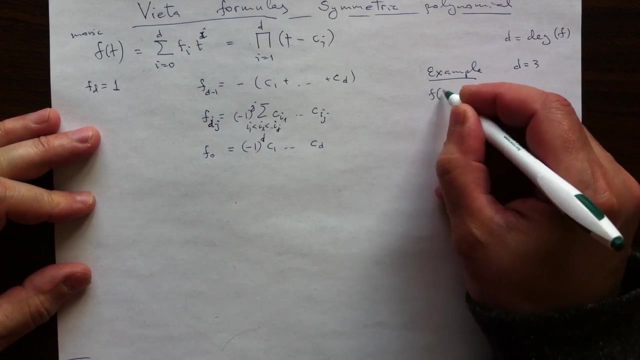 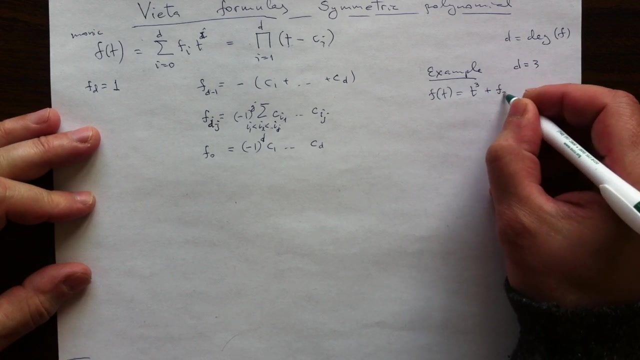 all the way down to the last jth. so that is a generic form of a coefficient. these formulas are called Lieta formulas after François Liet. for example, if t is equal to 3, our harmonic polynomial will look like t- cube plus some coefficient at f1t plus f 0. 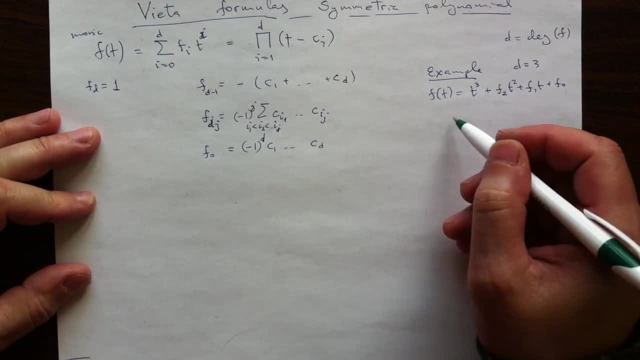 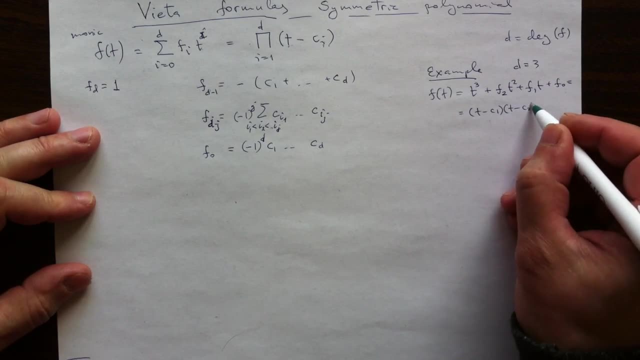 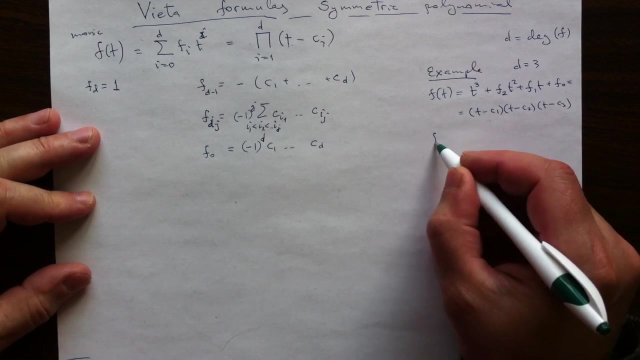 so that is a generic form of a harmonic polynomial. and then let's assume it's c1, c2 and c2 are half of the嗎. all right, C3 are its roots. So then what we can say about F2 is that it is. 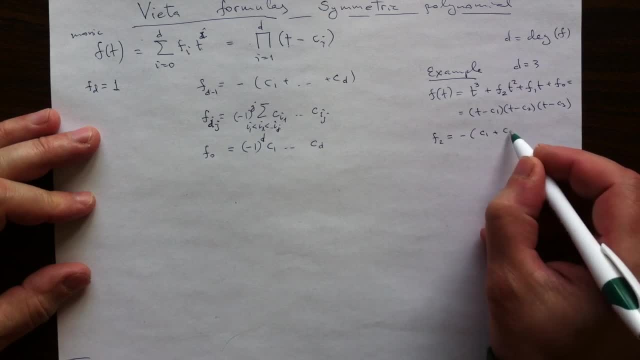 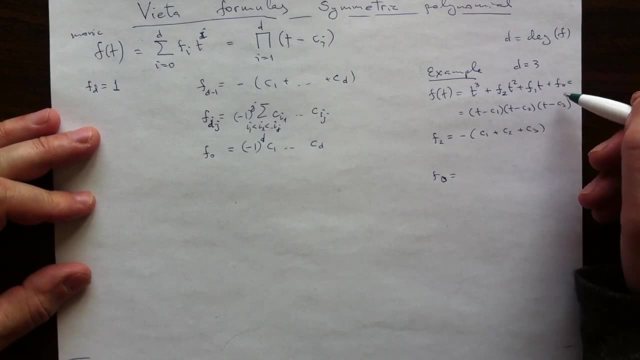 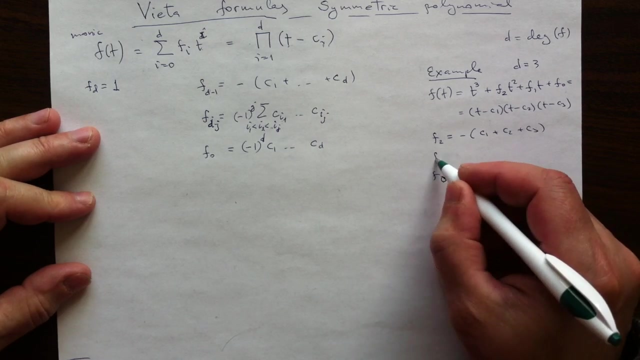 negative the sum of C1, C2, C3.. F3 is sorry. F0 is the product again with negative sign of C1, C2, C3. And the coefficient in between. F1 is positive. sum of. 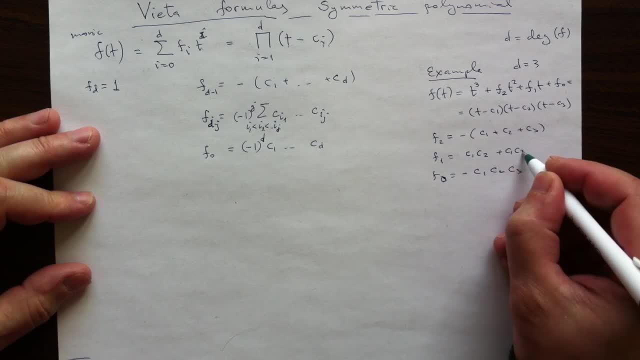 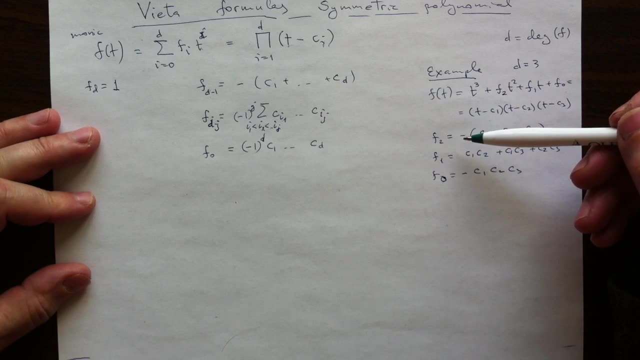 products of two: C1, C2, C1, C3, C2, C3.. And in general that is a feature of Viettis formulas that the sign changes if you progress along the list of your coefficients. So you start for the sub-leading. 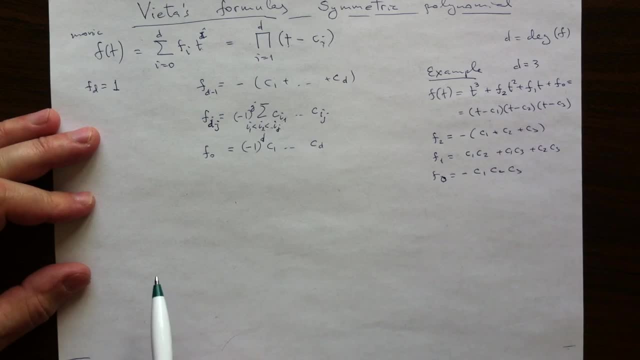 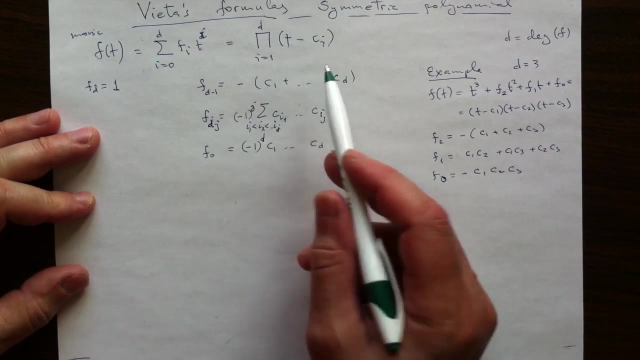 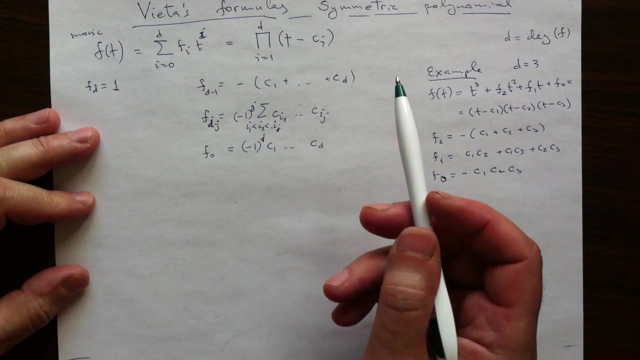 term. you start with minus, and then you go plus, and then you go minus, and so on all the way through. These expressions of coefficients as roots, these terms, expressions in terms of roots, are symmetric in this root, And that is of course inevitable because roots are all on equal footing. 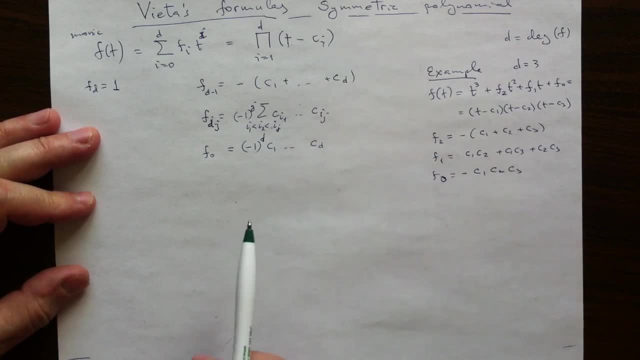 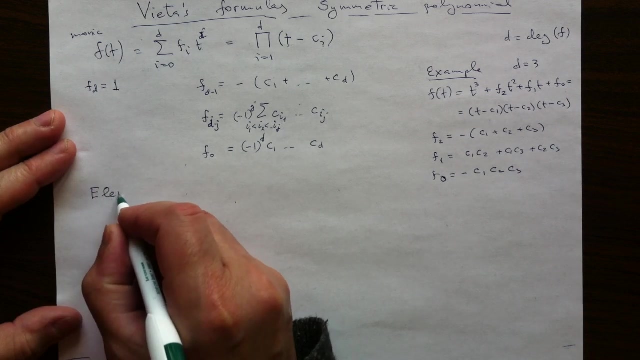 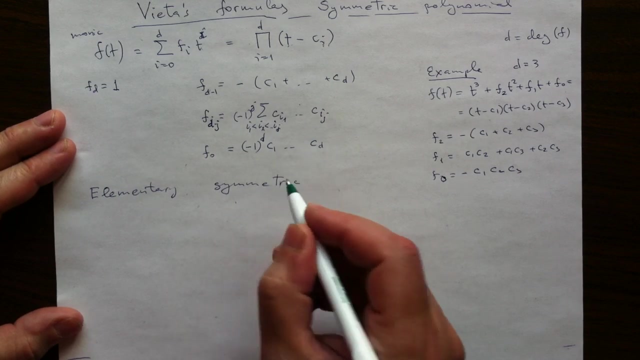 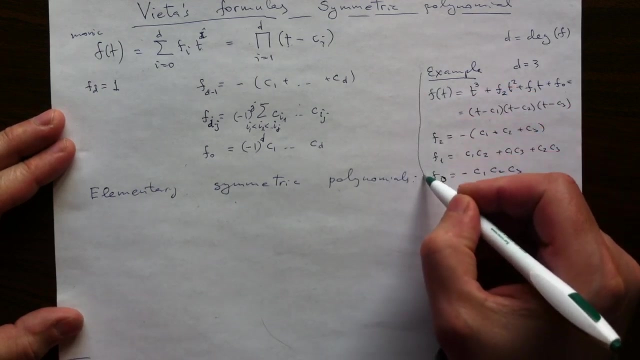 There is no root number 1 and root number 2.. It's our choice. It's an artificial numbering of them, So they're all on equal footing. All the expressions containing them have to be symmetric. In elementary, symmetric polynomials are those expressions. 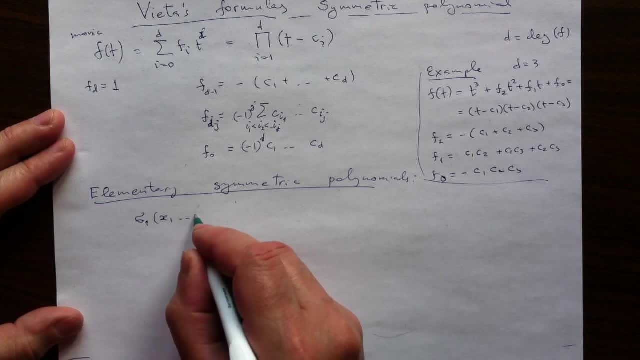 sigma 1 in x1 up to xd will be just the sum of the of the. these are nodes. Sigma d, the very last on that collection of variables, will be the product of all of them And all are nodes, And all the way through in between, so say. 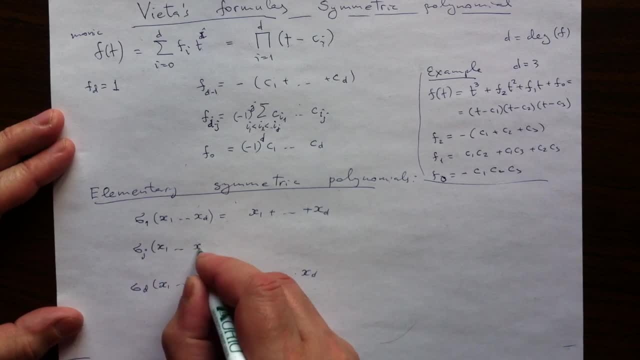 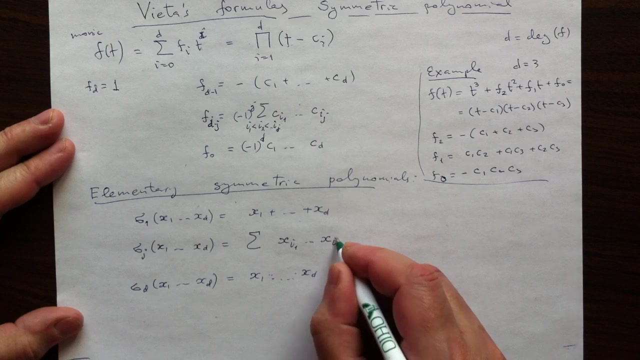 sigma j of x1, xd is the sum of two times all possible products of j, copies of the variables. but all the variables will have to be different and that is assured by disordering, and each such product is appearing once. So these are elementary symmetric polynomials. What is 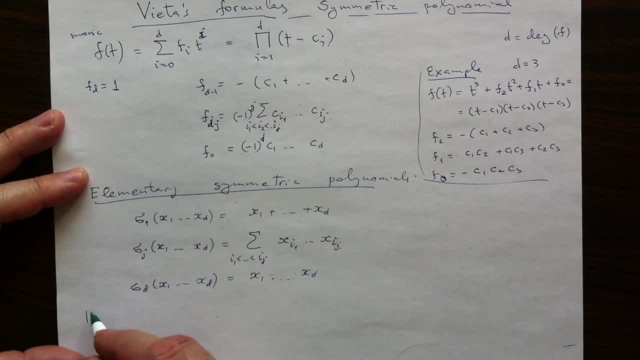 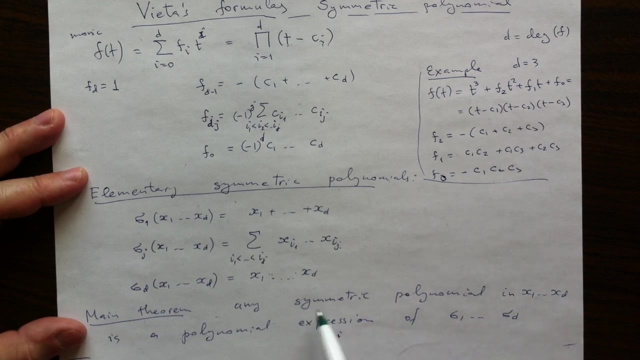 so special about them. This is the main theorem on symmetric polynomials. Any symmetric polynomial in these variables, x1 up to xd, is in its own right a polynomial expression of this elementary symmetric polynomials. Moreover, it is possible to write an arbitrary symmetric polynomial as a polynomial of these sigmas only.